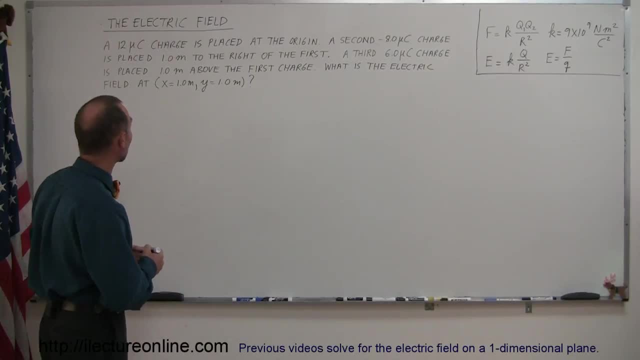 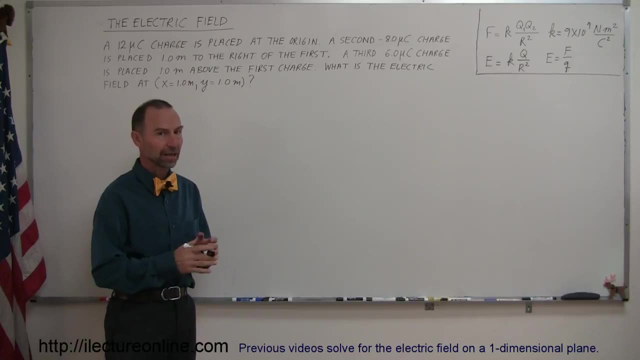 Welcome to iLecture Online, and here's another example of how to work problems dealing with electric field. This time we're going to look at something a little bit more complicated. We have multiple charges, not on a straight line, so this is a two-dimensional problem. 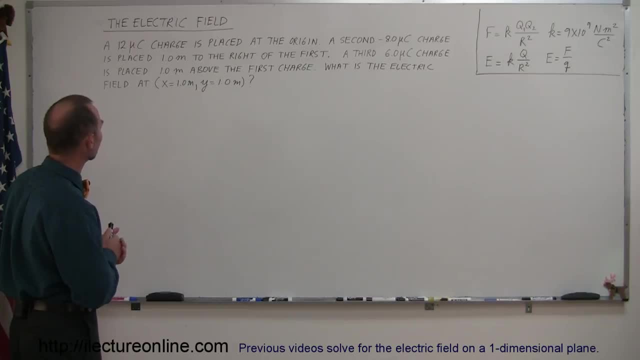 Let's take a look at this problem. It says here that we have a 12 microcoulomb charge that is placed at the origin. We have a second minus eight microcoulomb charge placed one meter to the right, and then we have a third, six microcoulomb charge that is placed one meter above the. 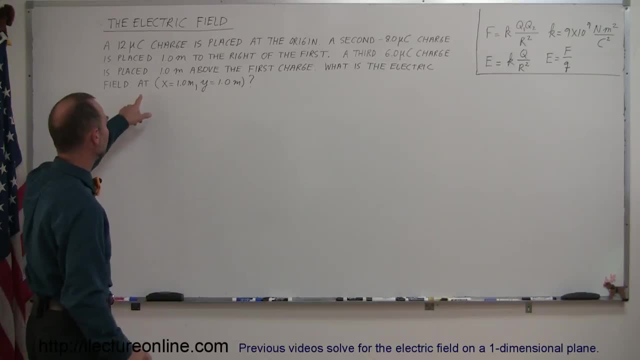 first charge? and what is the electric field at a location where x equals one meter, y equals one meter. So let's draw a diagram of that, using xy plane, to get a feel of what this problem is all about. So there's our y-axis and there's our x-axis. Let's place our charges. We have a 12. 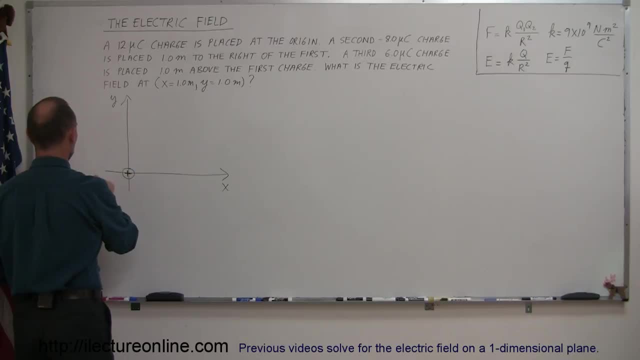 microcoulomb charge. right here It's a positive charge. so we go: q1 equals 12 microcoulombs. We have a second charge placed to the right right here That's a negative charge. that's at a distance of one meter. 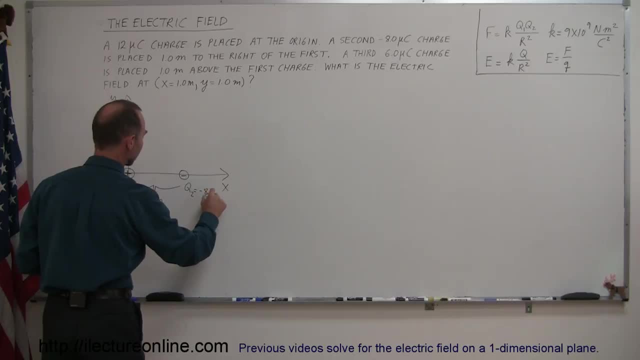 and call this q2, and that's equal to minus eight microcoulombs. And then we have a third charge which is placed directly above the first charge. one meter above. That's going to be another positive charge, and that's q3, and that's equal to six microcoulombs. 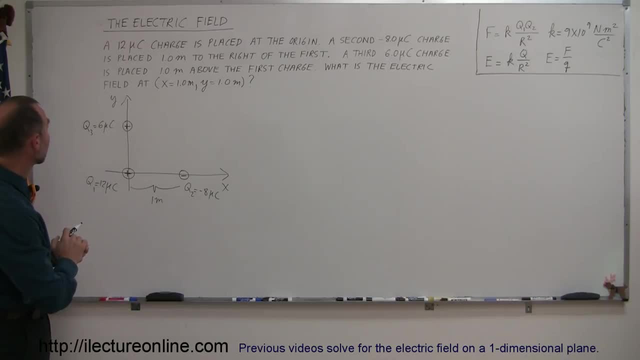 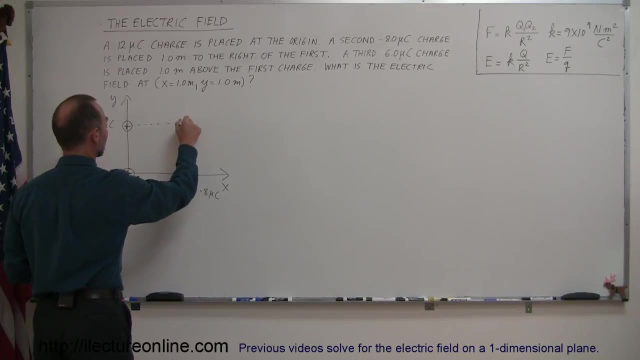 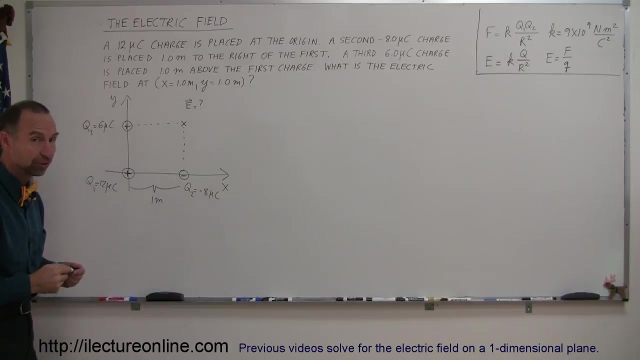 All right, now we want to put find the location of interest, which is, if we complete the square here, it looks like it's right at this location. We want to know what the electric field is at this location. All right, due to the presence of those three charges. Okay, where do we start? That's. 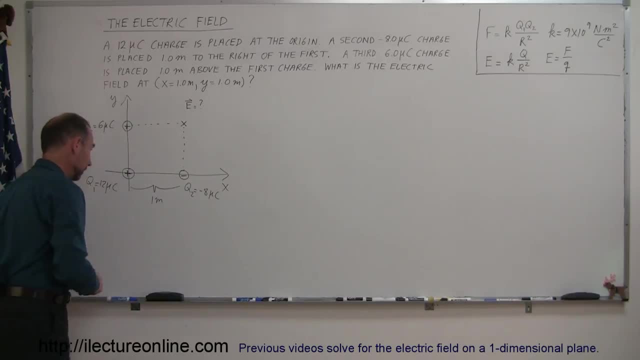 always the difficult part. and if you're at this point wondering where to begin, always grab a color pen and draw the electric fields graphically at this location due to the presence of these other three charges. that way you get started. you get more of a visual, more of a visual picture. 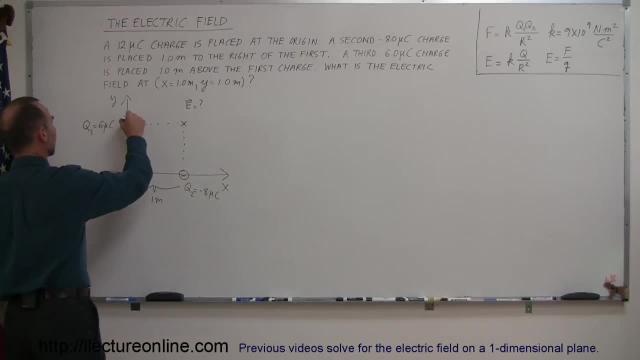 of what this problem is all about. remember that for positive charges, the electric fields are in the direction away from the charge. for negative charges, the electric fields are in the direction towards the negative charge. and here that's again. that's a way for the positive charge, so that sometimes helps determine. 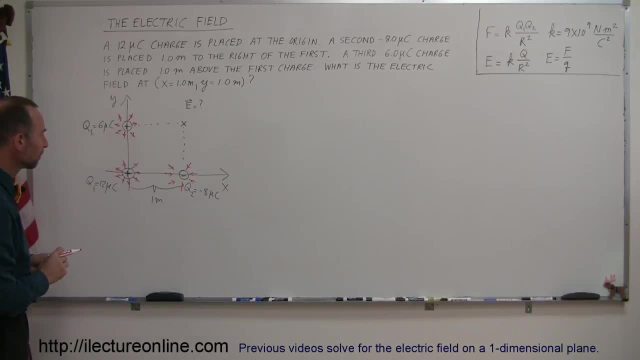 what the electric field direction will be at any place on this plane. so now we look at this location right here. we go one charge at a time. i guess i will go this direction for the first charge being a positive. what's electric field direction over here? due to discharge and it. 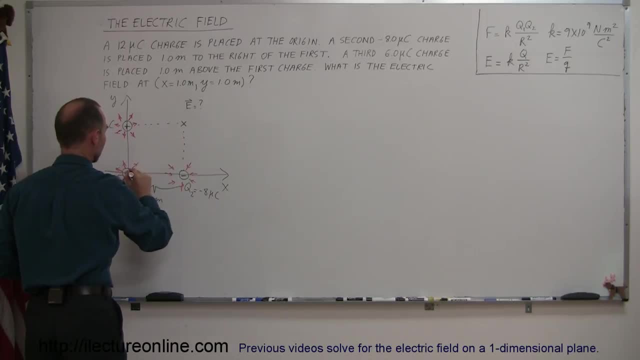 looks like it should emanate in this direction, so diagonally, straight across the electric field should be like this. so this would be e1, the electric field due to charge. one. now we go to charge two fields are in the direction towards the charge, so e2 should be down this way. call this e2. and then finally, due to discharge- right here. 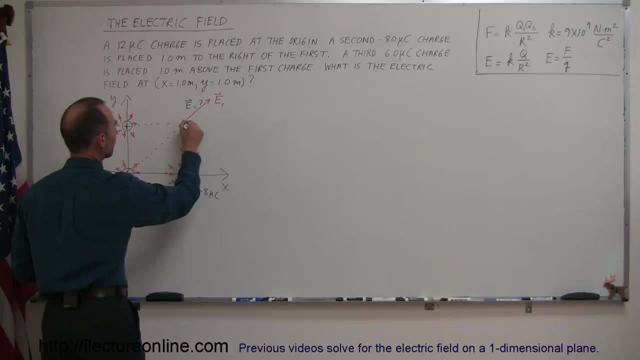 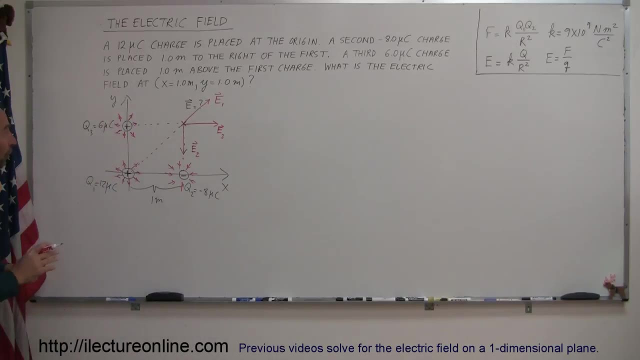 the field will emanate away from this, so the e3 would be in this direction. all right, so now we've identified the three electric fields caused by the three charges from at this particular location, and now, of course, to find the net electric field, we need to do a vector sum of those three electric 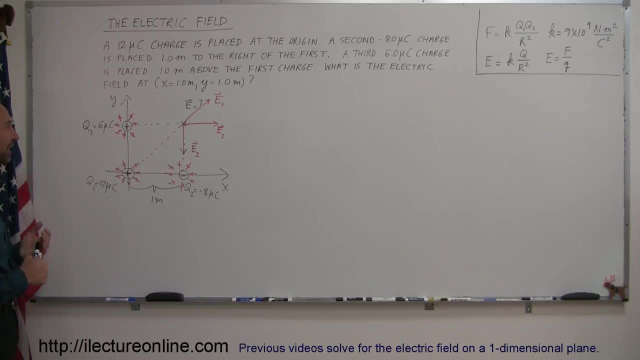 fields. now, of course, with vectors, if we do vector sum, we need to find the x and y components of each vector and, of course, before we do that, we need to find the magnitudes of each vector. so let's start now. the next step is find the magnitude of each of those three vectors. so e1. 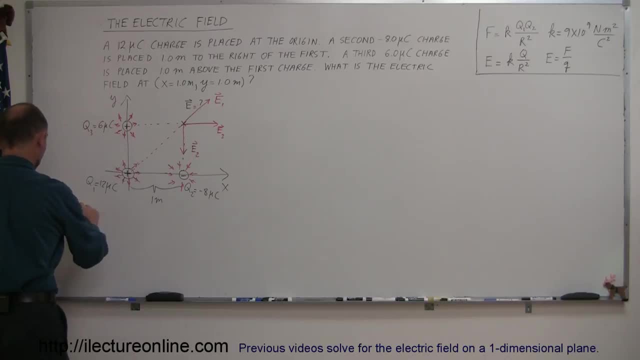 is equal to: and again, since it's a magnitude, let's draw some absolute values around it. we only care about positive values here because we just want to know the magnitude. so it's equal to k times q1, over the distance from q1 squared. plug it in the numbers. this is: 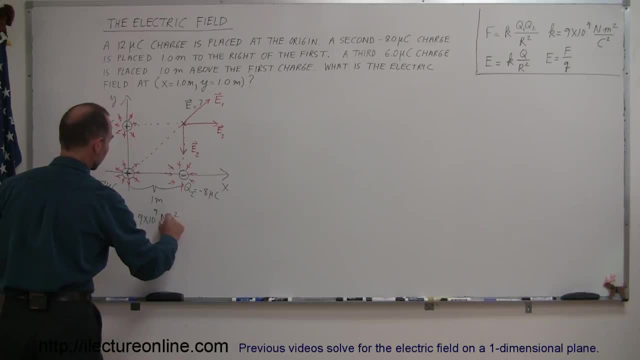 nine times ten to the ninth newtons meter squared per coulomb. squared times q1. q1 is 12 microcoulombs, which is 12 times 10 to the minus 6 coulombs divided by the distance squared. Now notice that this is the diagonal of a square that's one meter by. 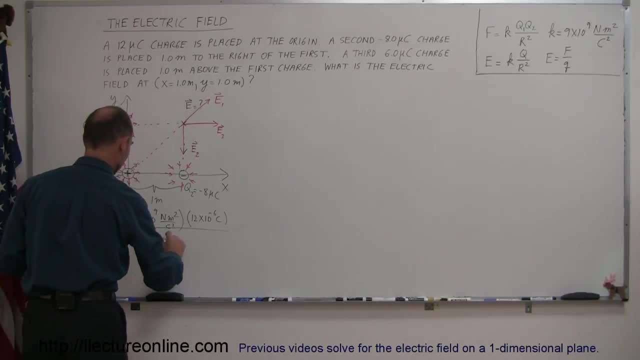 one meter, which means that this is the square root of two. the distance across would be the square root of two meters, and then we have to take the square root of two meters and square that which, of course, is equal to two meters squared Alright. 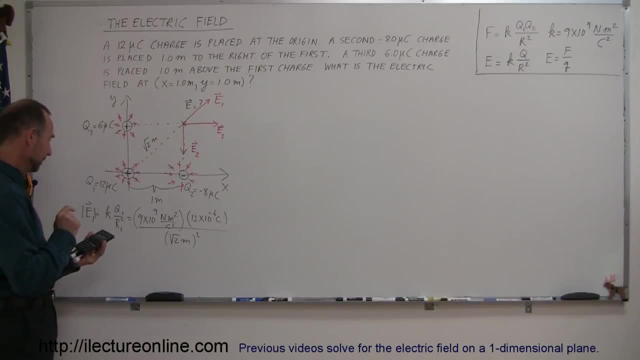 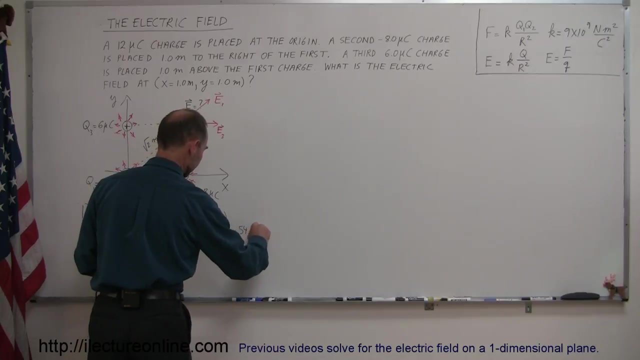 gram-meter calculator. I got one right here. Let's see here: nine e to the nine times 12, exponent six minus equals, and then divide that by the square root of two. squared that's divided by two and I get 54,000 Newtons per Coulomb. So that's the 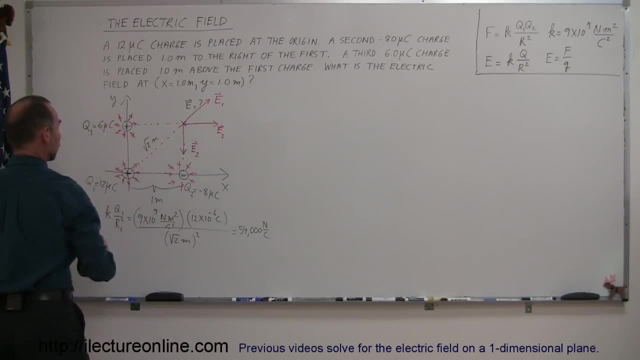 magnitude of the electric field at this location due to discharge right here, and of course we already know that the direction is outward. but right now we don't worry about that. Second magnitude, the magnitude of E2, due to the presence of Q2, so that's k Q2 divided by the 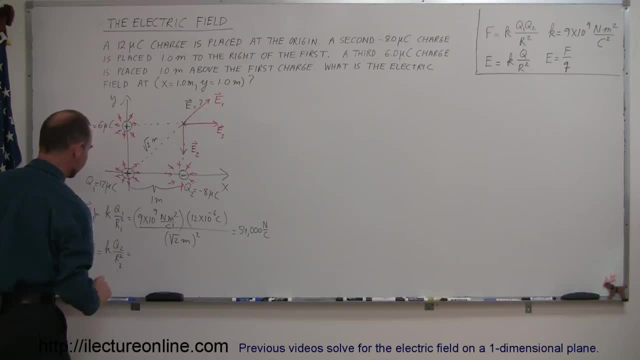 distance from Q2 squared, that's equal to playing the numbers nine times ten- to the ninth Newtons meter squared per Coulomb squared multiplied the times. now, even though it is a negative charge- I'm dealing with discharge right here- negative. 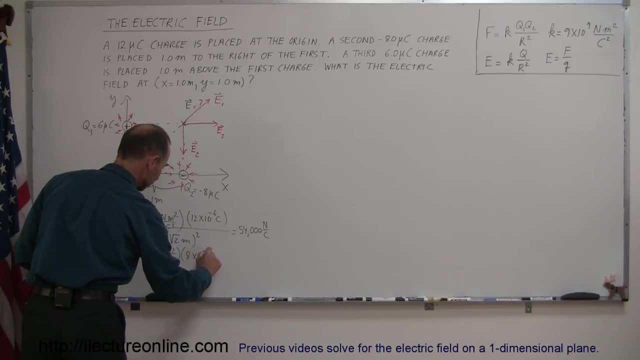 charge. we just put in the positive eight times ten to the minus six Coulombs, because we only care about the magnitude, all divided by the distance squared, and near the distance from there to there is one meter. so that's one meter squared. all right, using our calculator, what is that equal to? 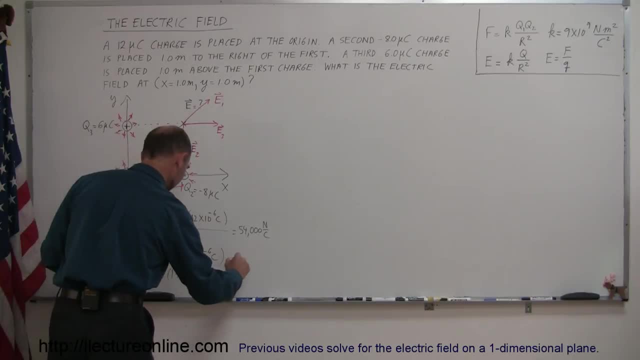 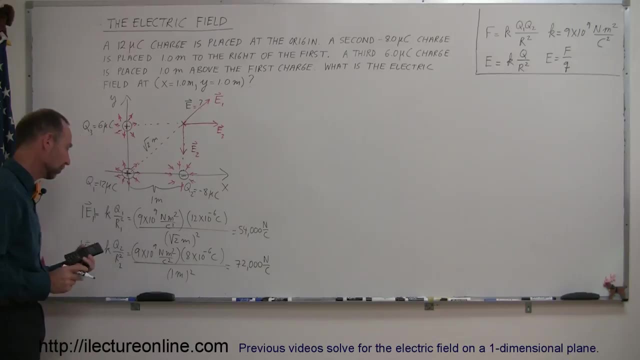 i don't even need a calculator, basically what i have there. if you punch things out, it looks like this would be 72 000 newtons per coulomb, because eight times nine is 72, so that looks like 72 000. uh, 10 to the mine, 10 to the 9th and 10 to the minus. 6 is equal to 10 to the third. 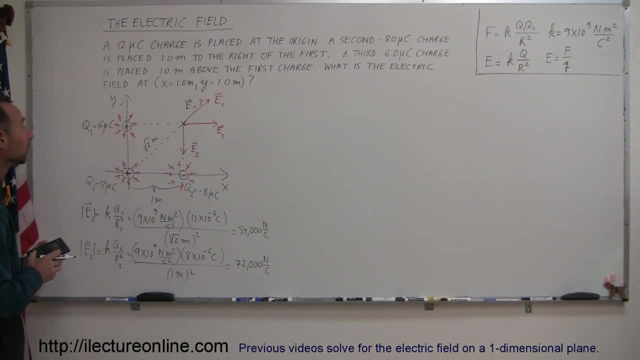 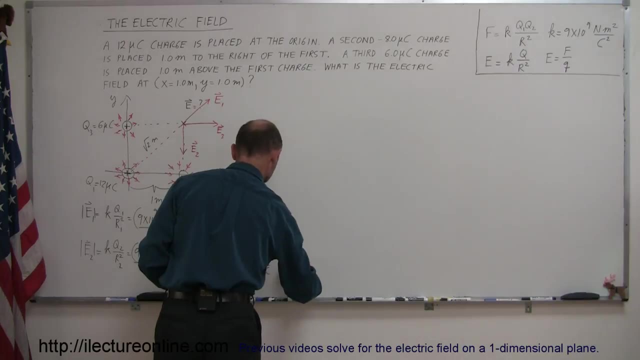 so the three zeros. so there we have the magnitude of e2. we need the magnitude of e3, and since i'm out of room, then here i'll plug. put it in right there. so e3 is equal to k- q3 divided by r sub 3. 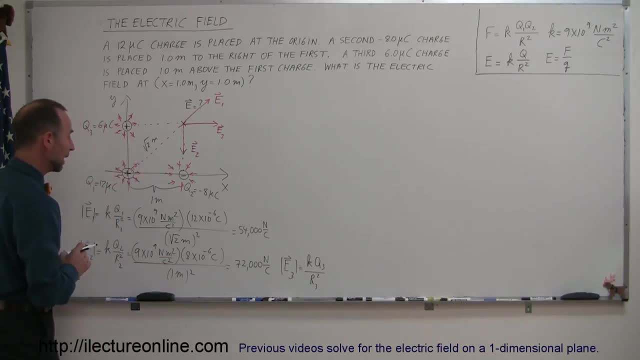 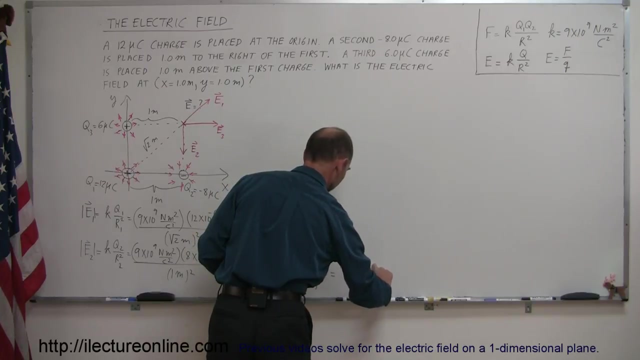 squared again. r sub 3 would be the distance between q3 and the point of location right here that we're interested in, and this is one meter. so q? r3 would be one meter. plug it in the numbers. this is equal to nine times ten to the ninth newtons meter squared per coulomb squared. multiply that times the size. 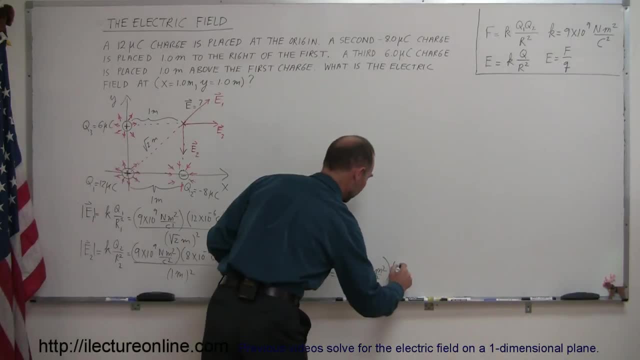 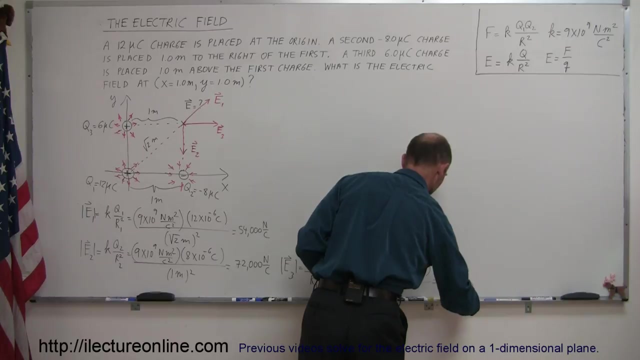 of q3, and q3 is six micro coulombs, six times ten to the minus six coulombs, and the whole thing divided by one meter squared, because the distance is one meter, all right, and six times nine is 54. so this would be 54 000 newtons per coulomb. so now we have the magnitudes. 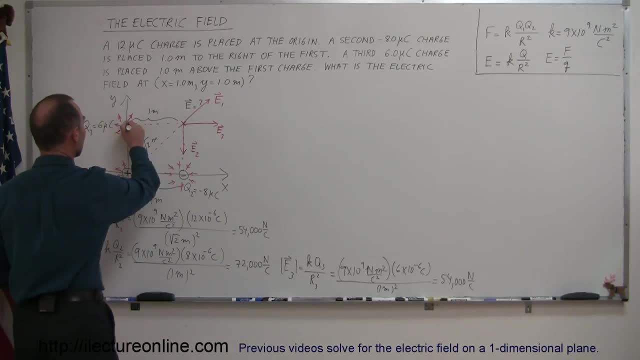 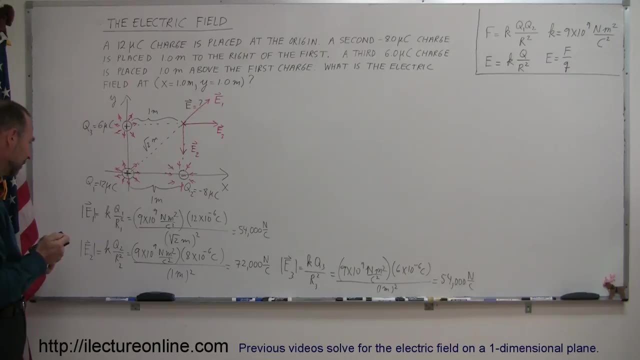 of all three electric fields at this location due to the presence of these three charges. so now we have to go ahead and add those together. but of course we cannot add them together algebraically. we have to add them together vectorially. that means we need to find the x and y components. 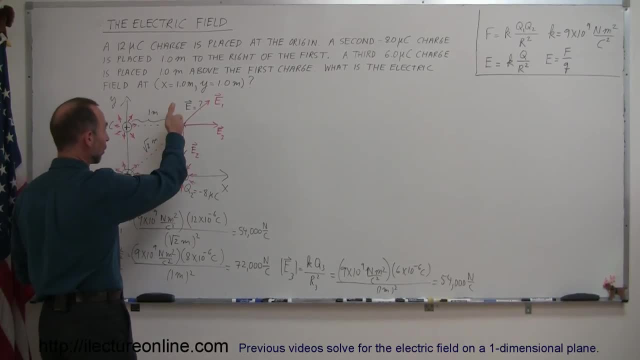 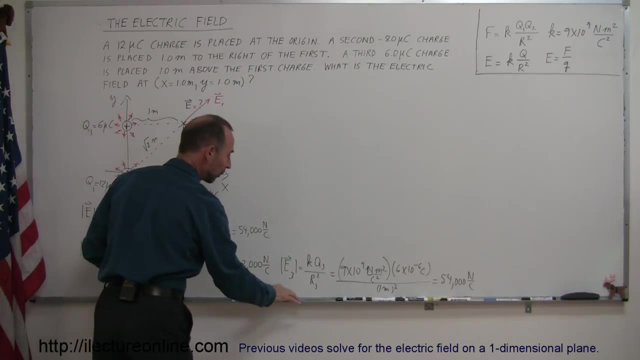 of each of the three vectors. now notice that e2 is already only in the y direction, e3 is only in the x direction, but e1. we're going to have to find both the x and the y components, looking for something with a slightly different color here. 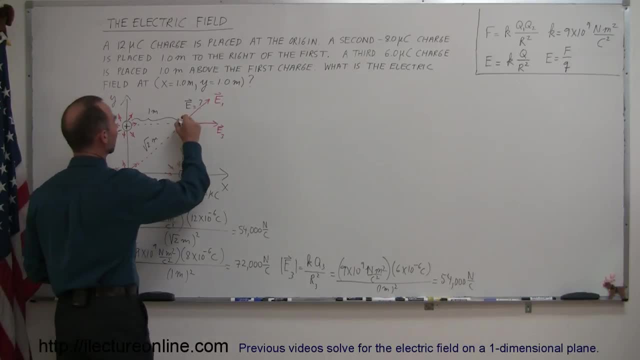 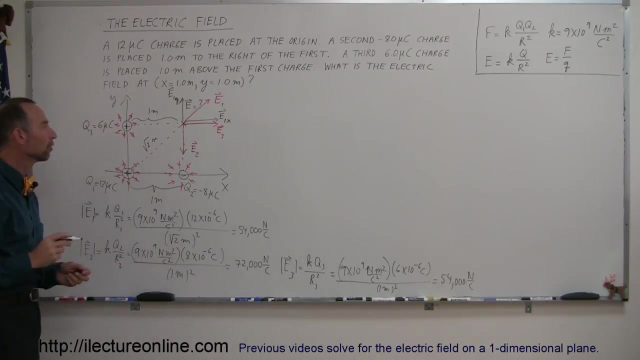 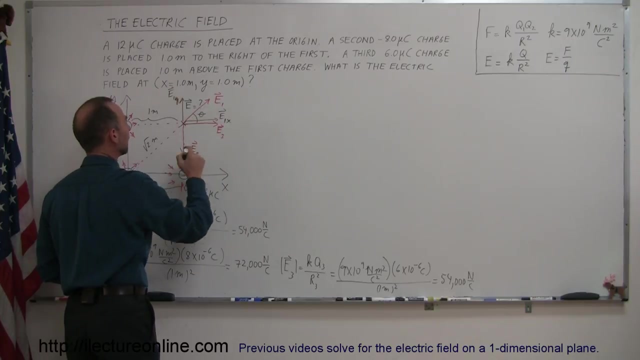 let me try, brown, see if that works. so i'm trying to find e1 in the y direction and i'm trying to find e1 in the x direction. there we go. those are the two components, the x and y components of e1. to do that, i'm going to need to know what this angle is. i need to know this angle here, theta. 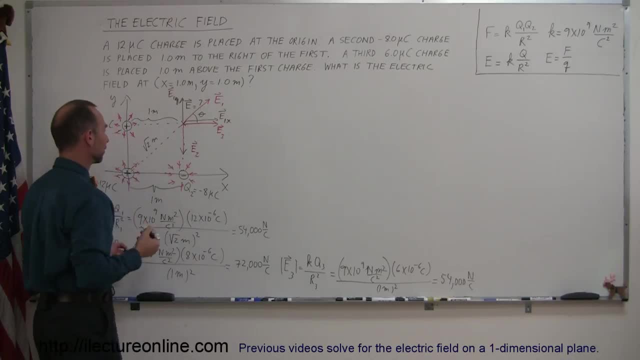 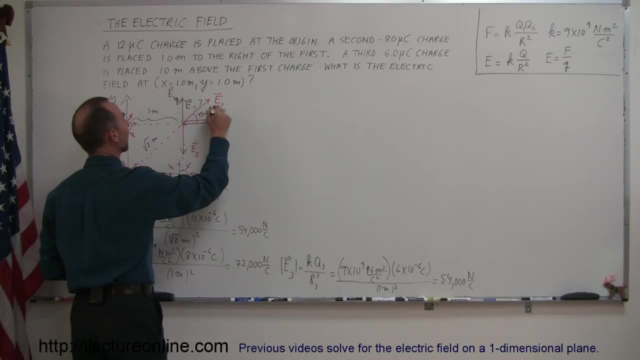 and of course, since this is a rec, not a rectangle but a square, it's indeed a rectangle, but it's a special rectangle. it's a square. all sides are the same. that means the angle here must be 45 degrees makes a little bit easier, so knowing the magnitude of e1. 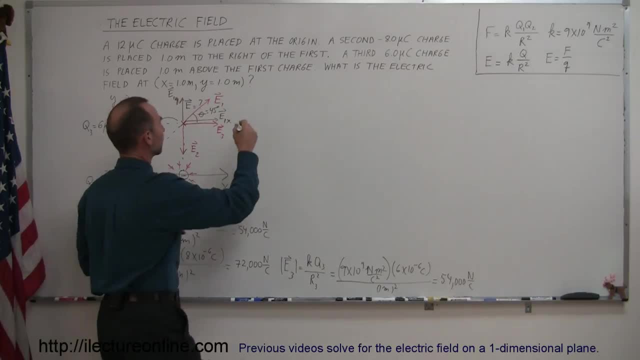 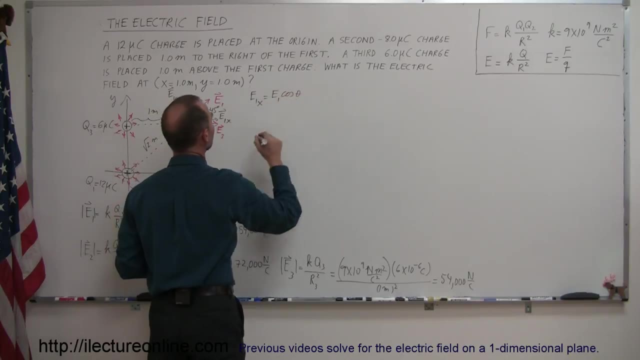 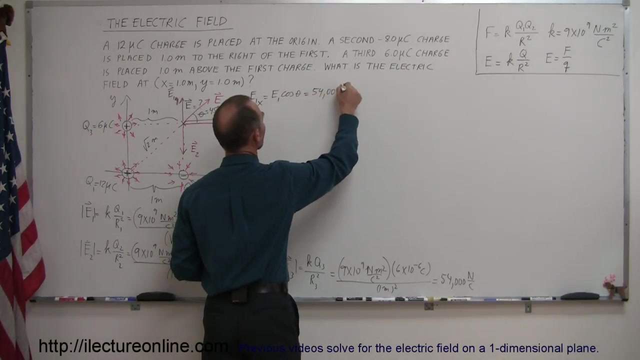 we can now find the magnitude of those components. so e1 in the x direction is equal to e1 times the cosine of the angle theta. the magnitude of e1 is 54 000 newtons per coulomb. we multiply that times the cosine of 45 degrees. 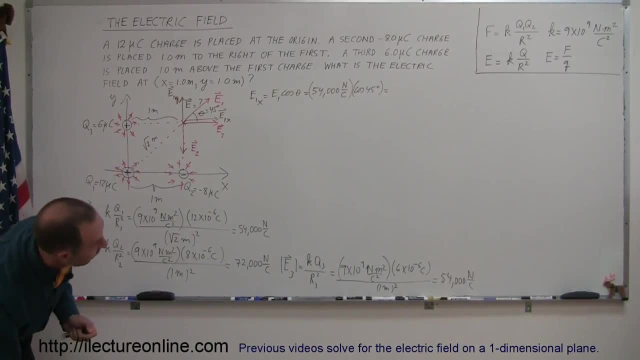 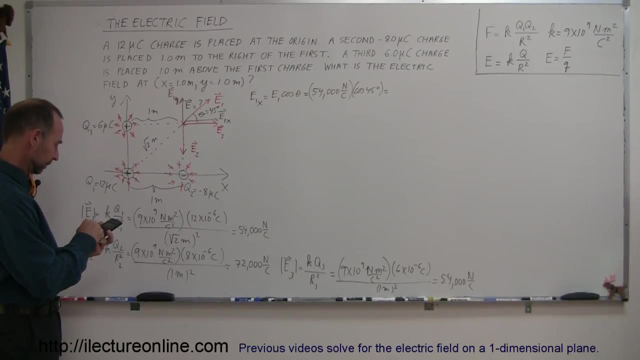 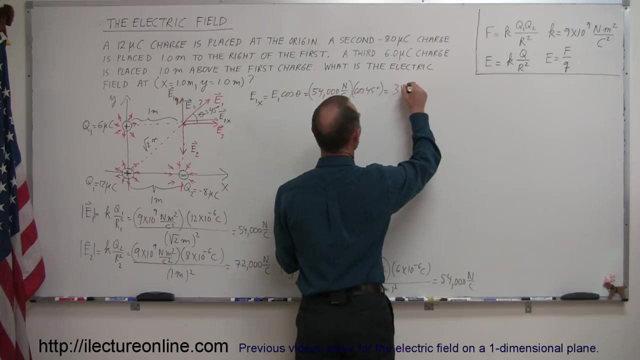 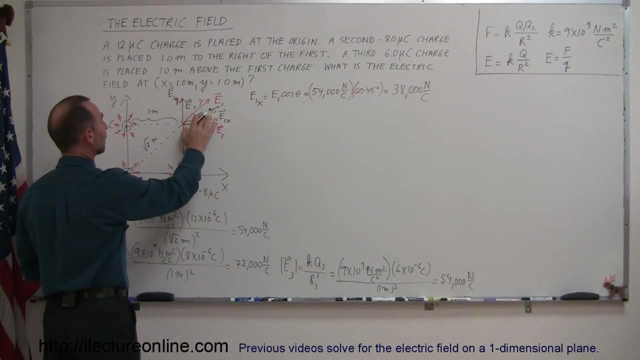 which is 0.707. what does that give us in terms of the magnitude of e1 in the x direction? okay, that's 38 000, i'm just going to round it off to 38 000 newtons per coulomb. and since the angle here is 45 degrees, that means the sine of 45 degrees is also 0.707. so we can then. 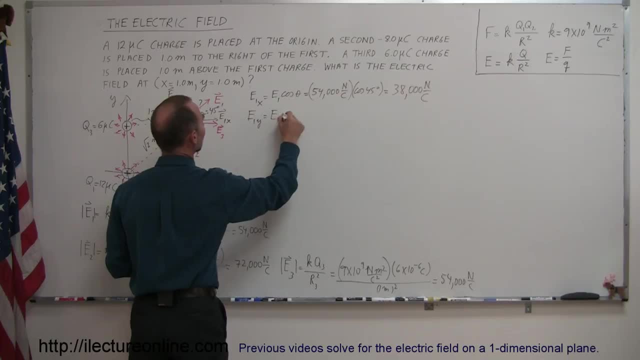 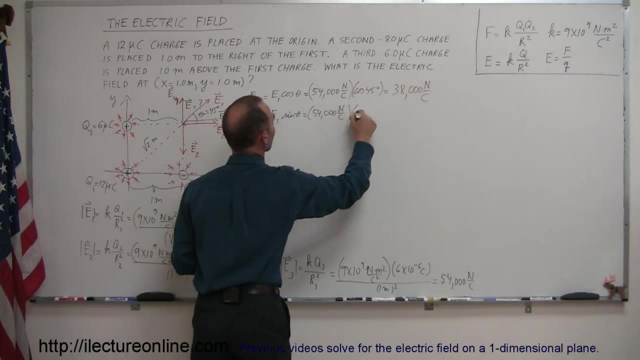 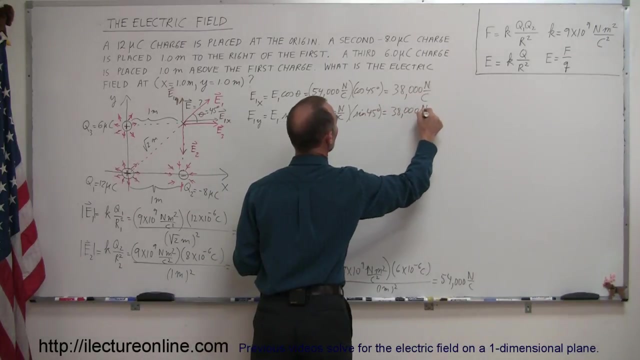 write that e1 in the y direction is equal to e1 times the sine of theta, or this is equal to 54 000 newtons per coulomb times the sine of 45 degrees, which is also 0.707 newtons per coulomb. all right, we're now ready to start adding these vectors. 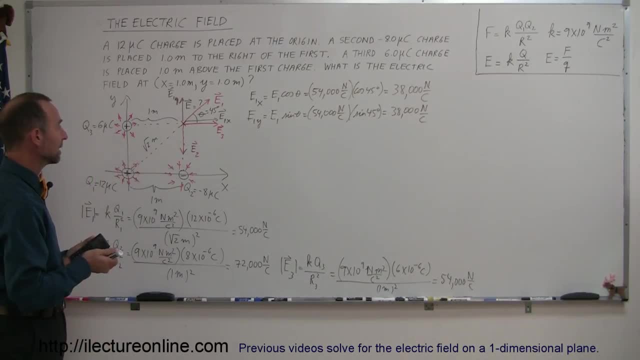 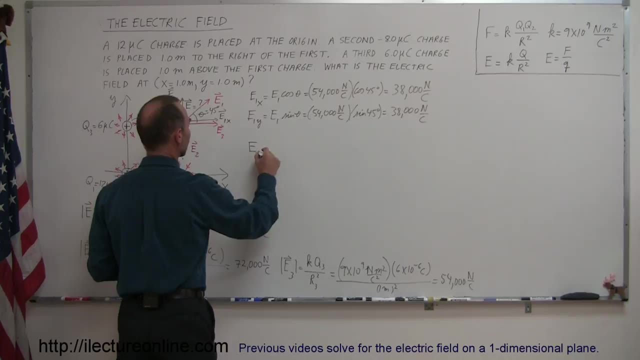 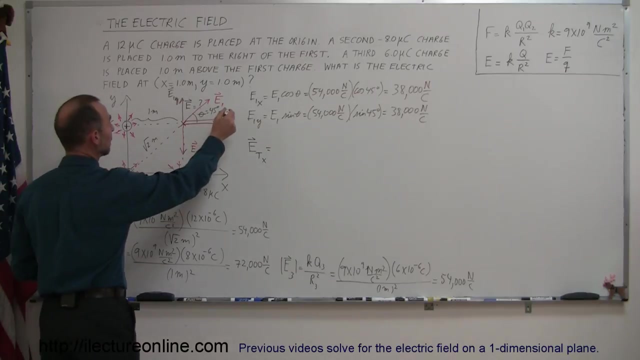 one direction at a time. so we're now going to find the x coordinate or the x component of the total electric field. so e total in the x direction is going to be the sum of all the x components. now let's find all the x components and we have an e1 in the x direction right there. so that's one. 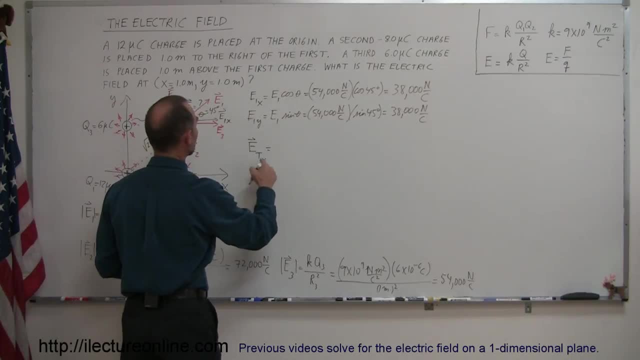 component and we have e3, so we're going to find the e1 in the x direction right there. so that's one component and we have e3. so e to the x direction is going to be e1 in the x direction plus e3, because the entire 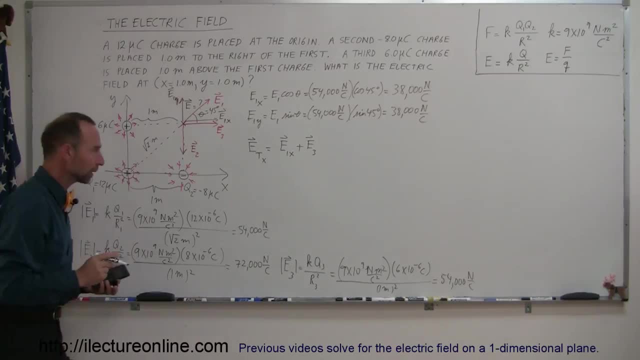 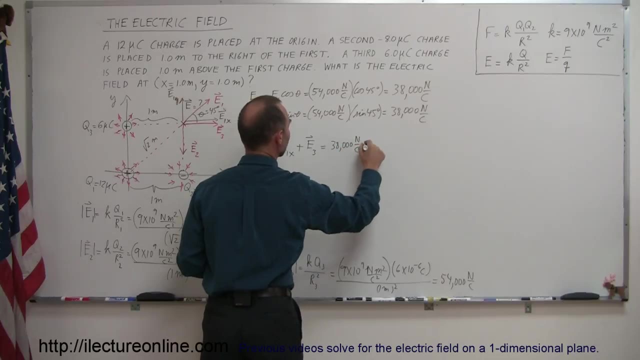 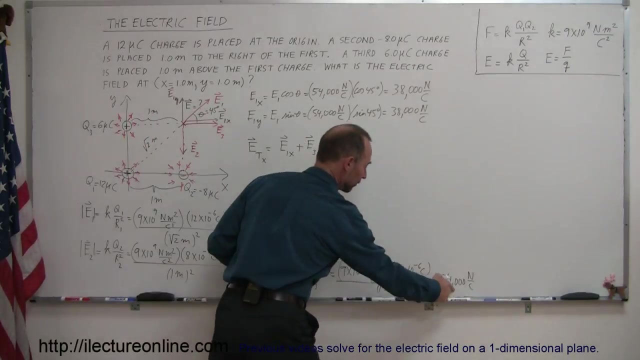 e3 is in the x direction. playing in the numbers, this is equal to 38 000 newtons per coulomb in the x direction. and e3? where's e3? it's right here. that's 54 000 newtons per coulomb, so plus 54 000. 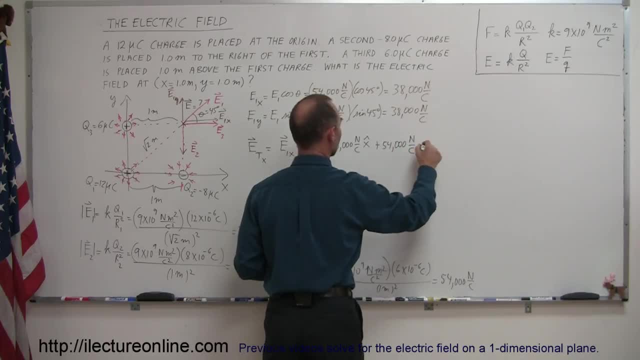 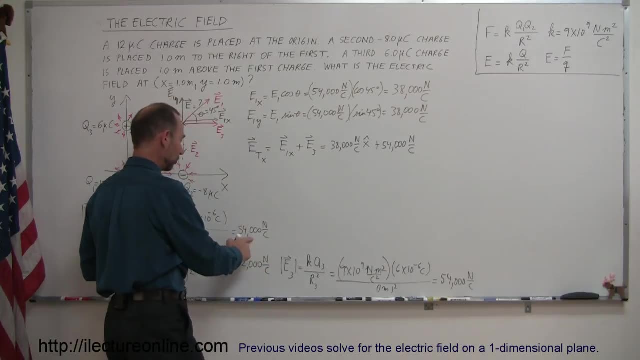 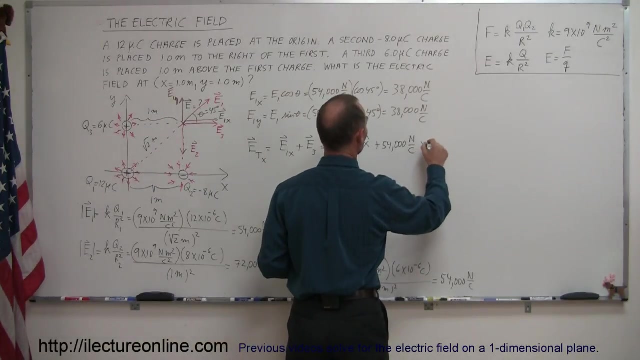 per coulomb and that is: hmm, wow, I just noticed the magnitude of E1 and E3 are the same. that just happened to be by chance. I just want to make sure I was doing this right. okay, Newton per coulomb, and that's also in the x-direction. 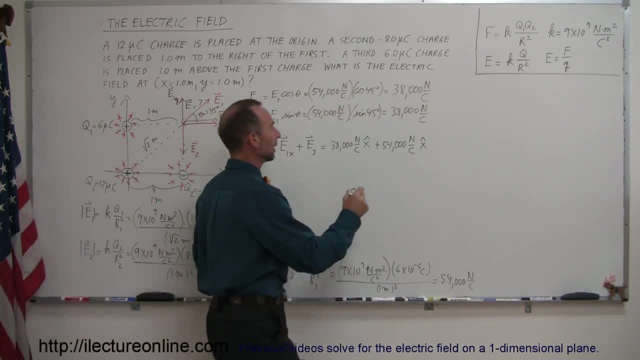 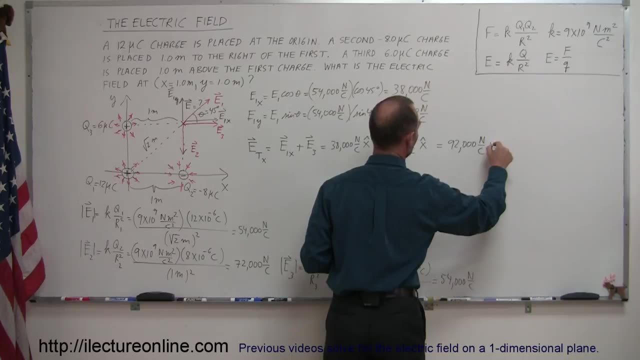 they're both positive because they both point to the right. so that means that E total in the x-direction is: that's 80,, that's 92,000 Newtons per coulomb, and that's in the x-direction. All right, so we now found the x-component of the total. 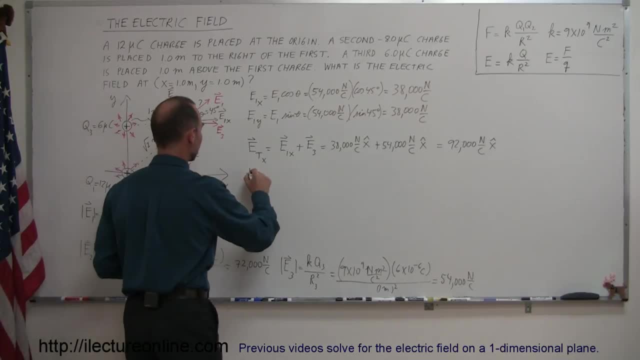 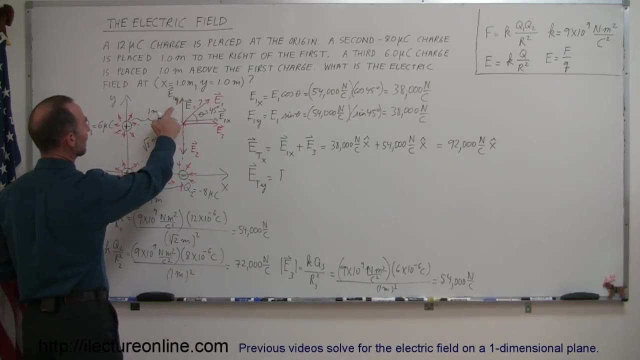 electric field at that location. I now want to find the y-component, E total in the y-direction and that's equal to E. well, let's see here what do we have? We'll have the E1 in the y-direction. that's the component in the y-direction. 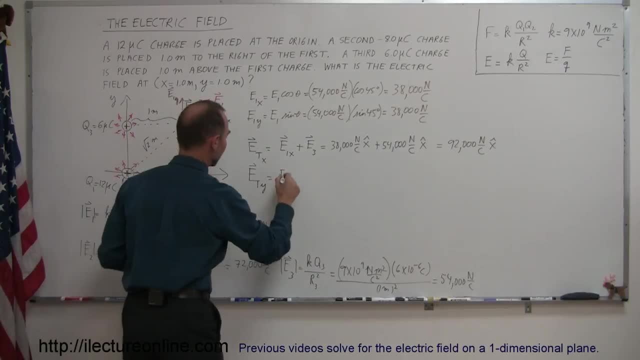 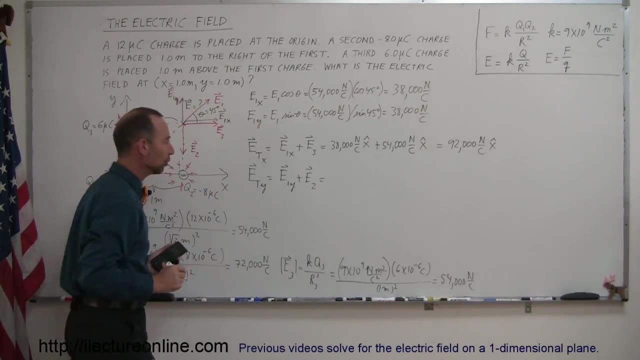 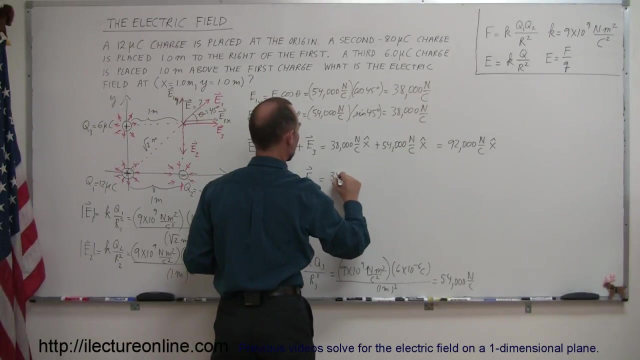 which is positive, and then we have E2, which is negative. so that means we add E1y plus E2, of course remember that E2 will be directed downward, it'll be a negative quantity. so this is equal to E1y, which is right here. that's 38,000 Newtons per coulomb in the 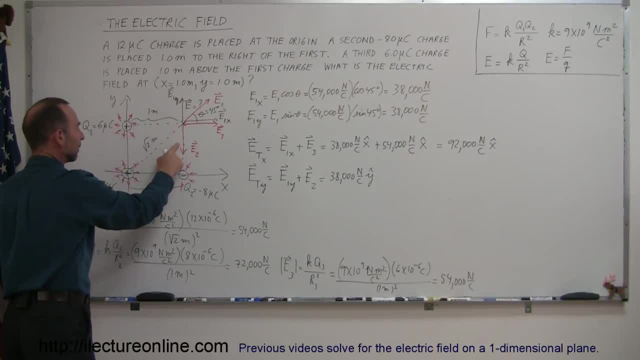 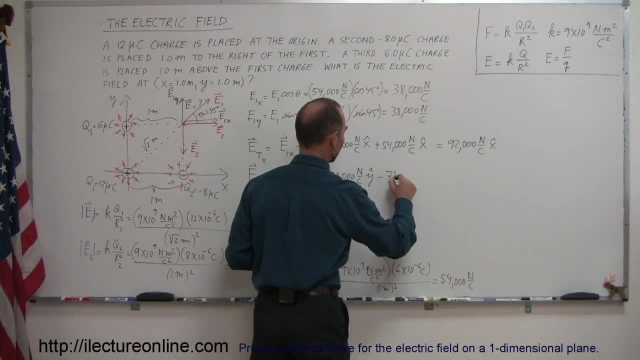 positive y-direction because it's pointing upward, and then minus E2, E2 is right here, 72,000 Newtons per coulomb. it's pointing downward, so 72,000 Newtons per coulomb in the y-direction. this makes it the negative y-direction and 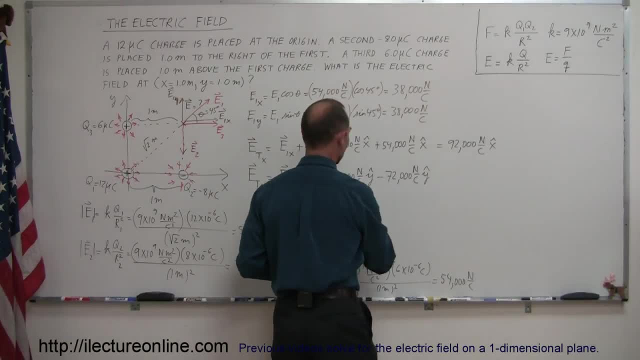 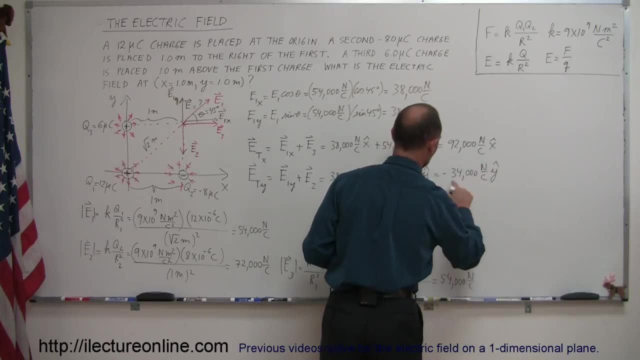 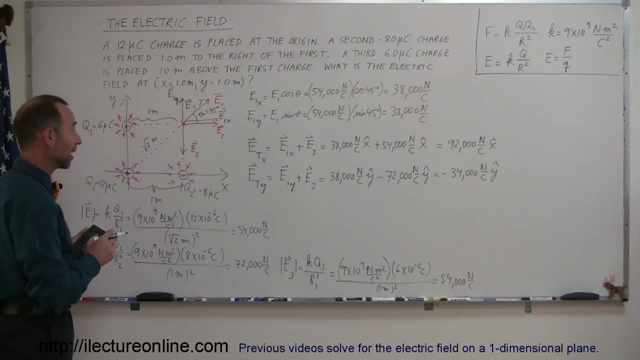 then that means the difference between those two is 34,000, so that's a minus 34,000 Newtons per coulomb in the y-direction. so this indicates it's a negative component. Alright, so far, so good. We have now found the x and the y components of the total electric field. 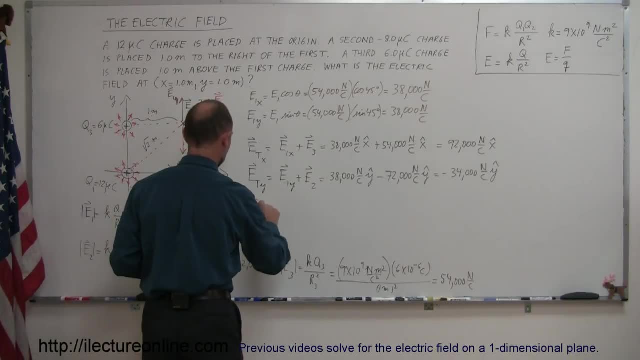 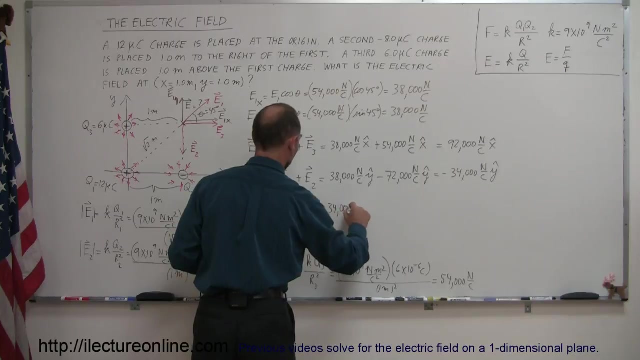 Now, of course, if we want to write this as a single vector, quantity E total is therefore equal to the sum of the two components. so that would be 92,000 Newtons per coulomb in the x-direction, minus 34,000 Newtons per coulomb in the y-direction. 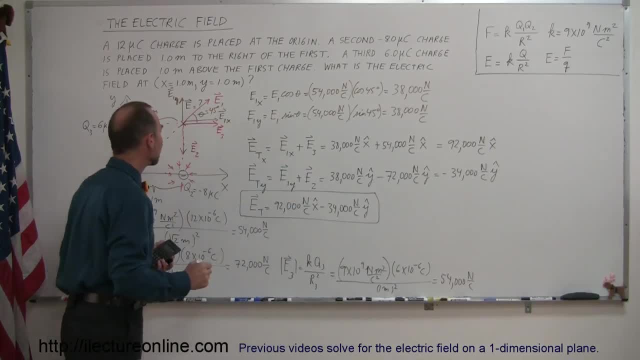 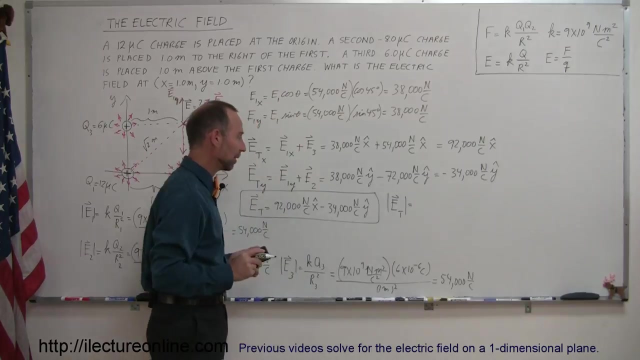 So this is the electric field at the given location due to the presence of these three charges. If you now want to find the magnitude of that, to find the magnitude of the total electric field strength, that would be written like that right. We put absolute values around it. the. 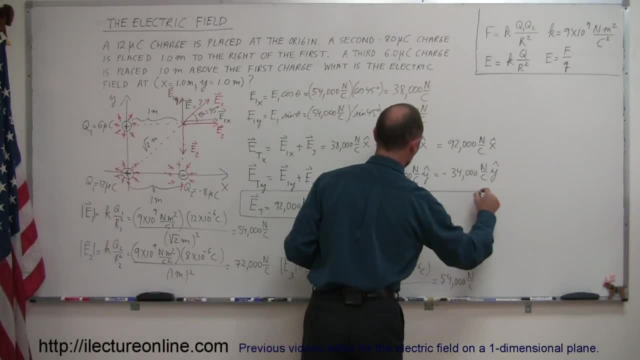 indicate the magnitude that is equal to the square root of the sum of the squares of the components. that would be E total in the x-direction squared plus E total in the y-direction squared And make it a little shorter here, so that's equal to the square. 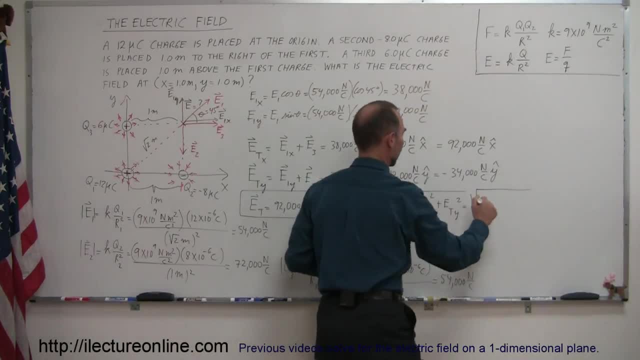 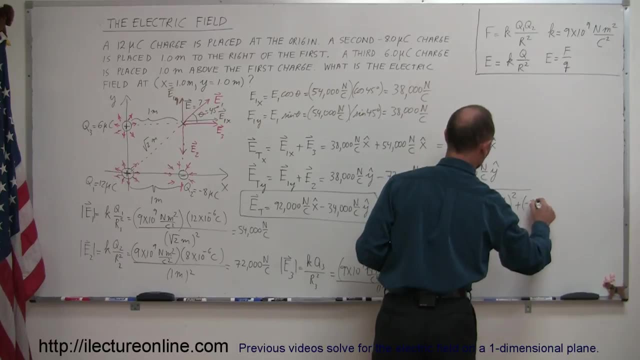 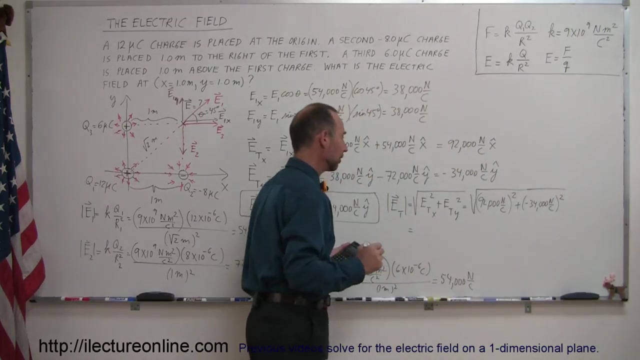 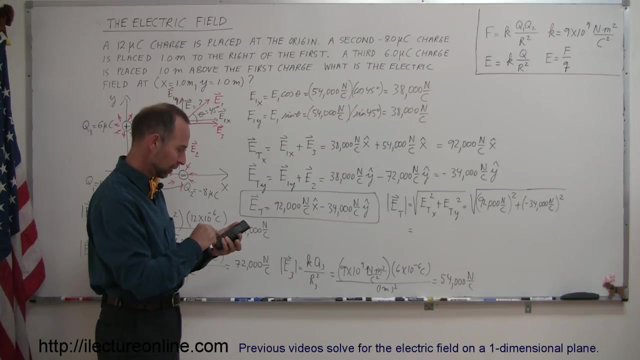 root of, and I'll take the two components. they're right here. so I take 92,000 Newtons per coulomb quantity squared plus a minus 34,000 Newtons per coulomb quantity squared and if I plug that into the calculator, so 92,000, we square that plus 34,000, we 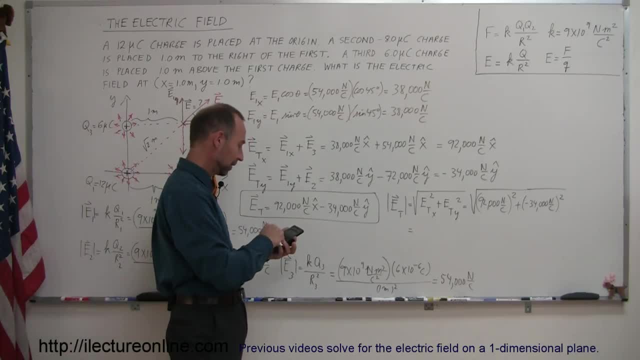 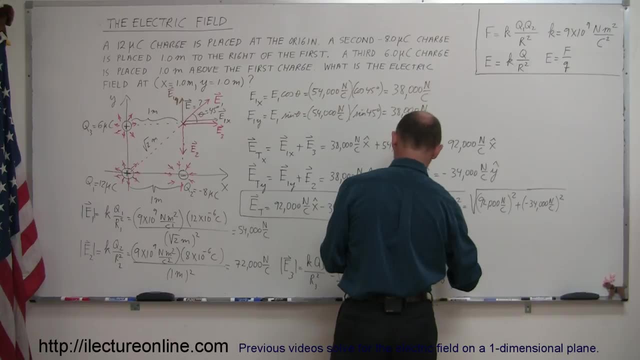 square. that doesn't matter if it's negative, because we're squaring it anyway. we add those two together, we take the square root and it looks like the total would be 98,000, round it off 98,000 Newtons per coulomb. so that's the. 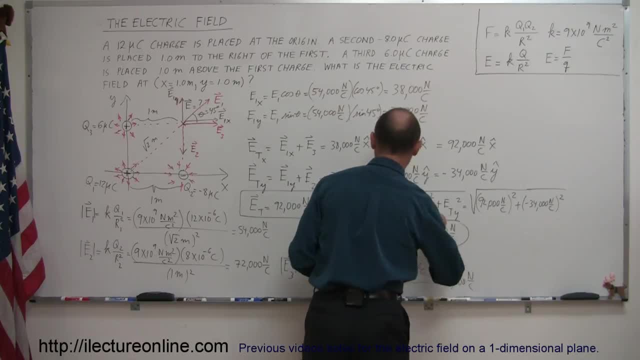 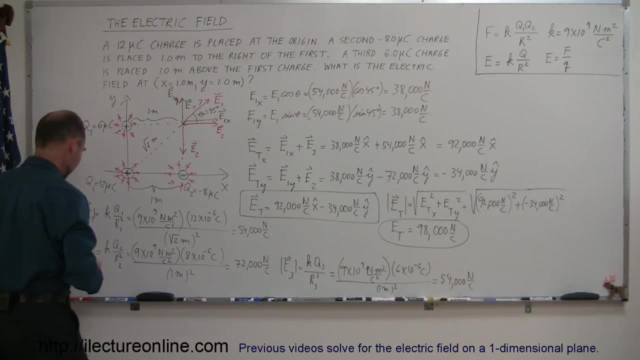 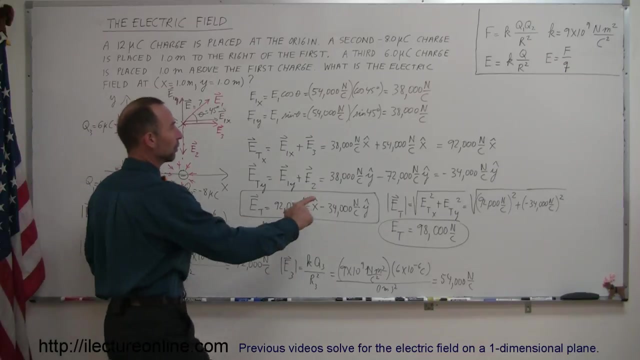 magnitude of the electric field strength. If you now want to know the direction of that, and let's at least put the components down here, let's try that out. so the final electric field has a positive component in the x-direction of 92,000 Newtons per coulomb. so that would be this vector right here. so 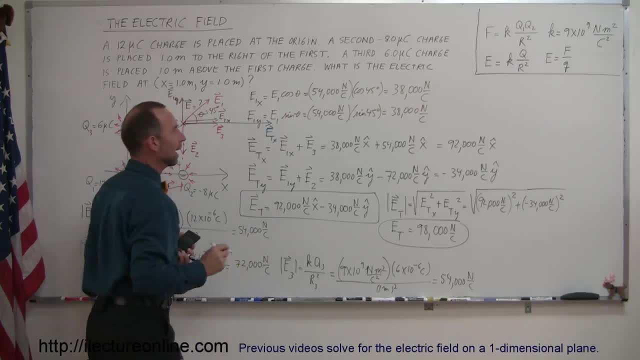 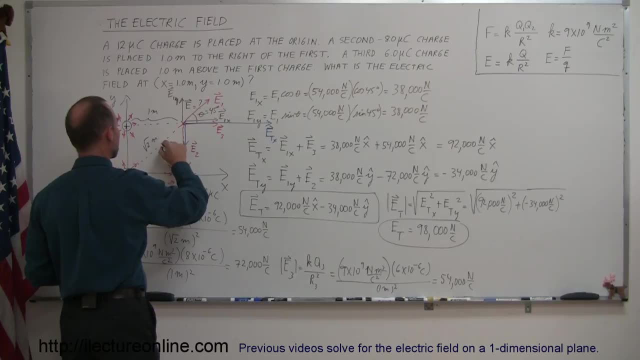 this would be E total in the x-direction. and then we have a component in the y-direction that's a minus 34,000, that would be this way, like here. so this would be E total in the y-direction. so these are the x and y components of the total, or sum of the. 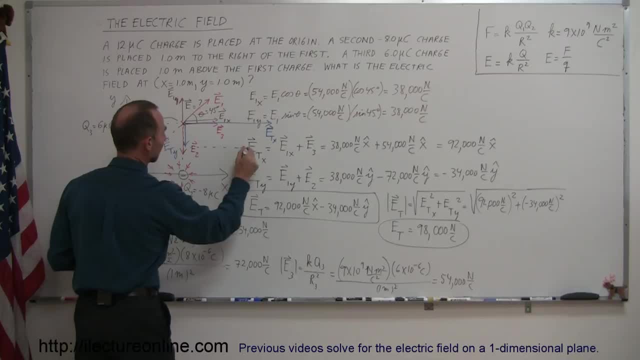 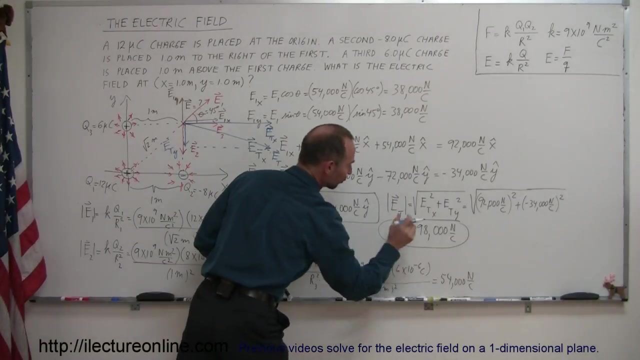 vectors and then, if you want to combine that, this would be then the vector representing the total electric field at that location due to the presence of these three charges. so the magnitude of this would be 98,000 Newtons per coulomb. 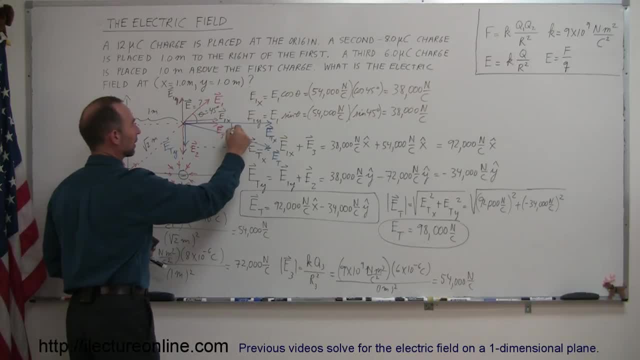 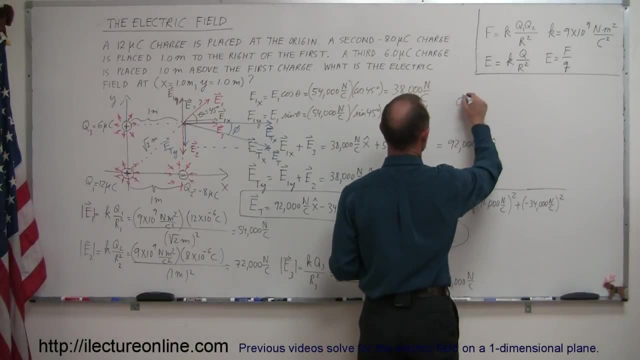 and then the angle, let's call it the angle. phi relative to the positive x-axis can be found by taking the arctangent. so we can say that phi is equal to the arctangent of the opposite divided by the adjacent side to that triangle. what I'm saying here is: 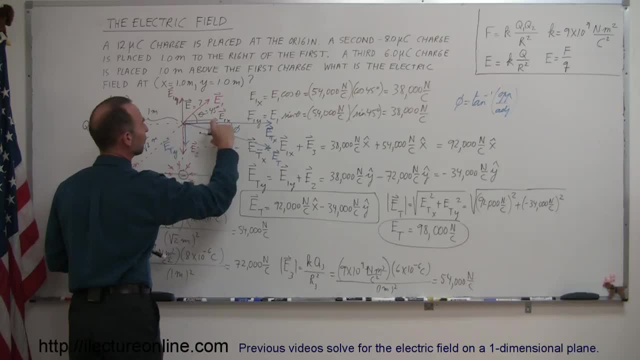 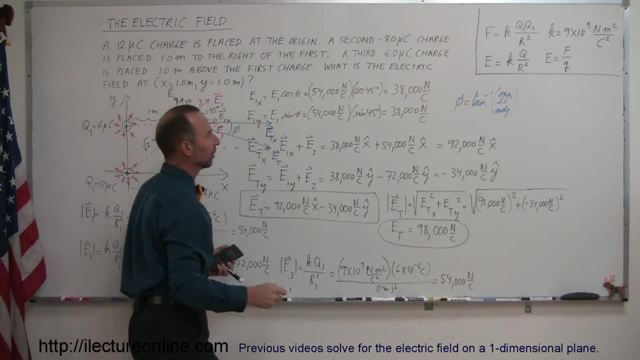 that this is the adjacent side to the angle. this would be the opposite side to the angle. so if we take the arctangent of the opposite divided by the adjacent, we get this particular angle. so in this case the opposite would be the y-component of the total, the y-component. 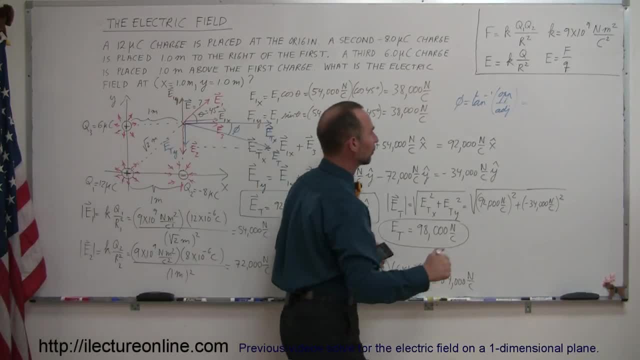 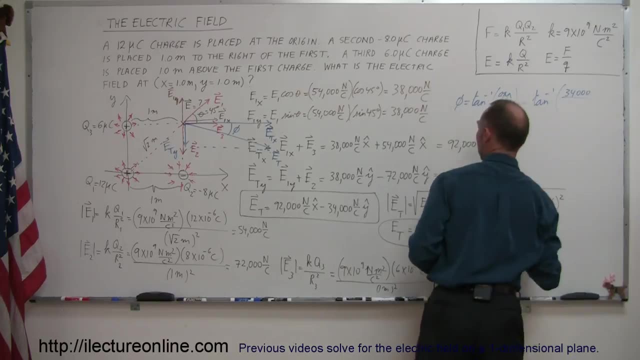 of the total. The y-component of the total right here is 34,000 Newtons. so that's the arctangent of the 34,000 divided by the magnitude of the adjacent side, that would be the 92,000, okay. 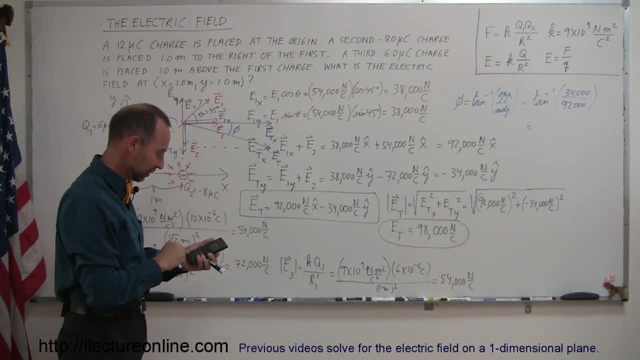 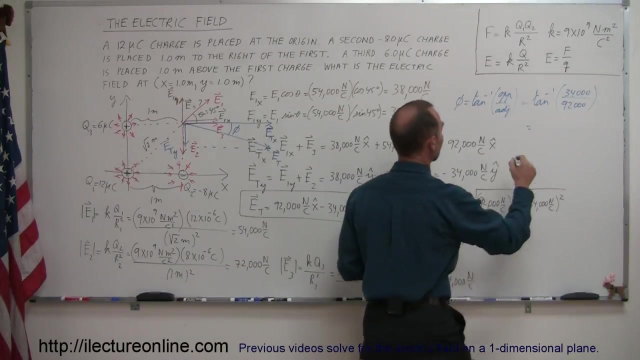 now the final answer here. we take 92,000 divided by- oh no, I'm sorry. the other way around- 34,000 divided by 92,000.. We take the arctangent of that and it's 20 degrees. 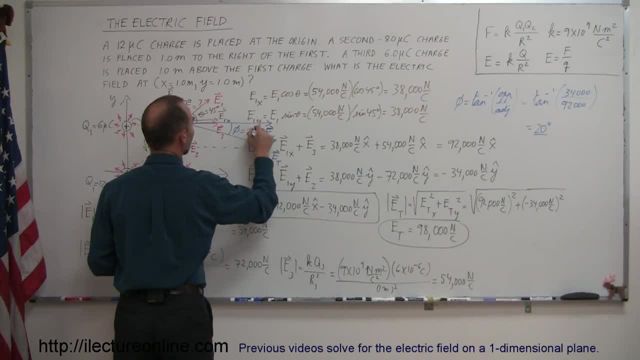 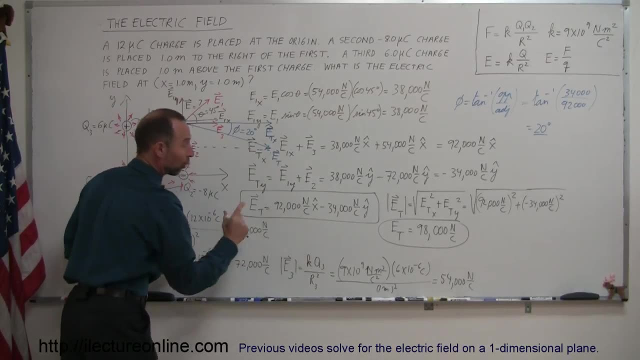 So now, finally, we know the full answer. We can either express the answer of the total electric field at that location in vector format like this, or we can do it by finding the magnitude and the direction relative to, in this case the positive x-axis. 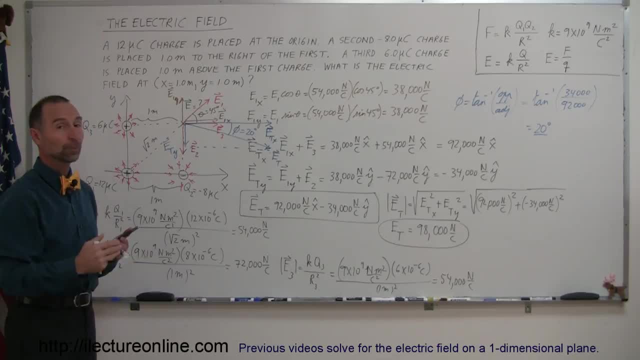 That's how you do one of these problems finding the electric field to the presence of charges, multiple charges that are not on a straight line. In this case it's a two-dimensional problem and you can see that's rather complicated, so let's go ahead and review it real quick. 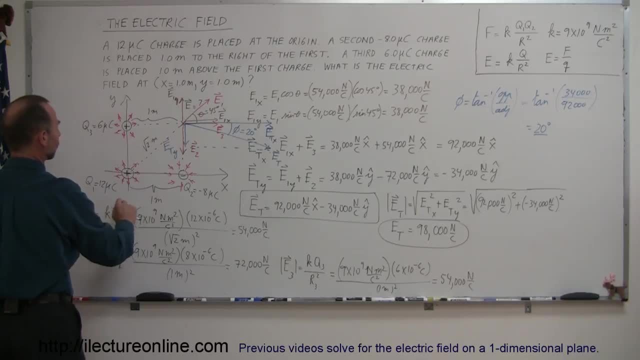 What we did was, initially, we drew a diagram of the situation, with the three charges placed in the correct location, and we found the location where we wanted to find the electric field. The next step, then, is to draw vectors representing the electric field. 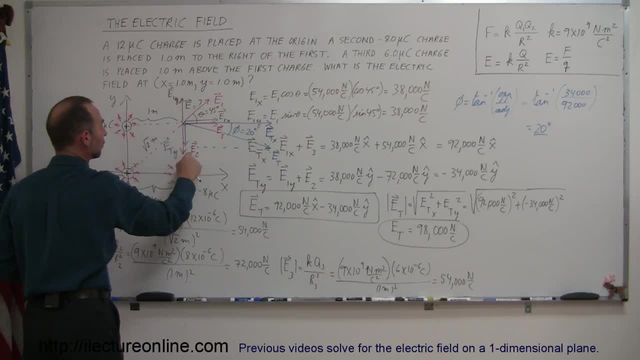 Okay, So we're going to draw the electric field and we're going to add the electric field to the presence of each of the charges, one at a time: E1,, E2, and E3, remembering that for positive charges, the vector field is away from the charge. 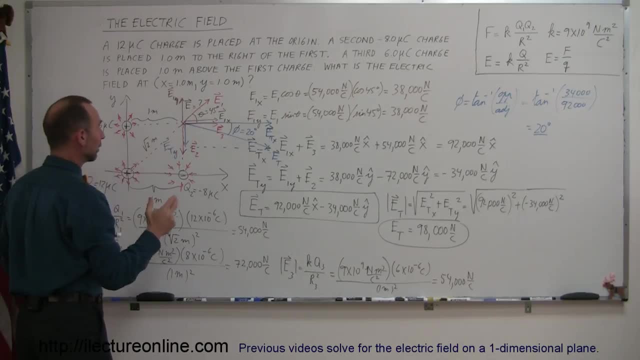 For negative charges, the vector is towards the charge. Then we need to add these together vectorially. To do that, we first need to find the magnitudes of the three vectors, which we did, and then we want to find the components, the x and y components of each of the vectors. 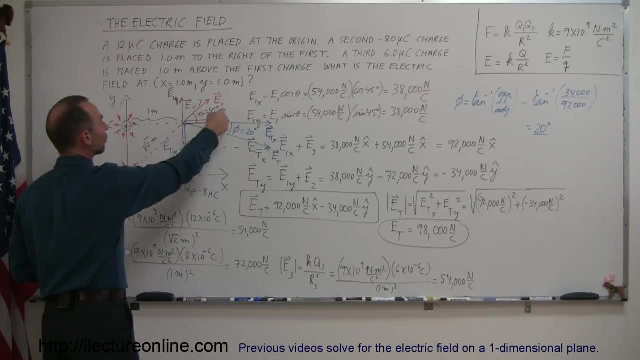 Now for E2 and E3, since they're already in the x and y direction, only not at an angle, we only have to find the components of E1. We use that equation, like that cosine and the sine, to indicate the x and the y components. 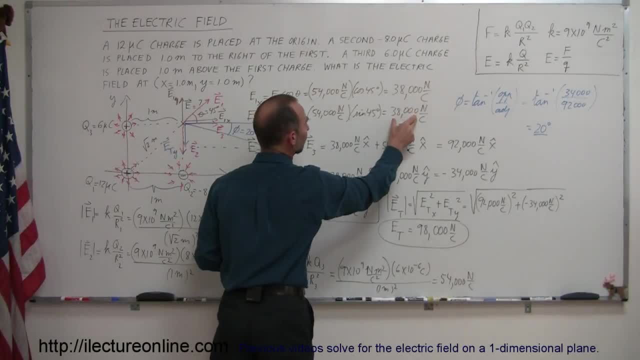 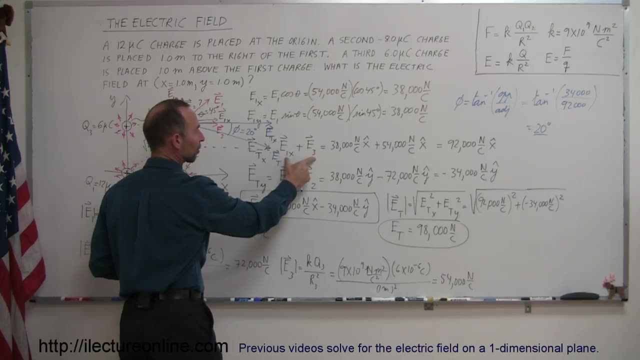 of that vector. Once we've found the magnitudes of those two components and the magnitudes of the other vectors, we then do a vector sum. E, total in the x direction is the vector sum of the x components of all the vectors and 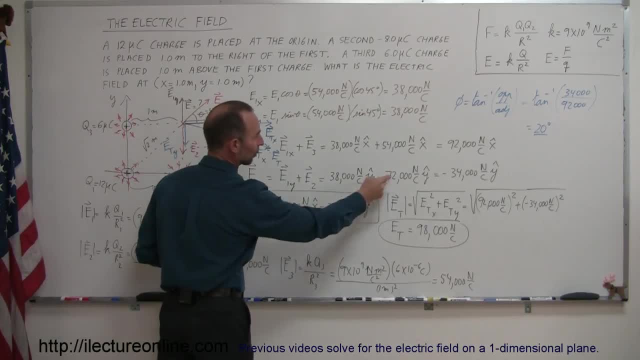 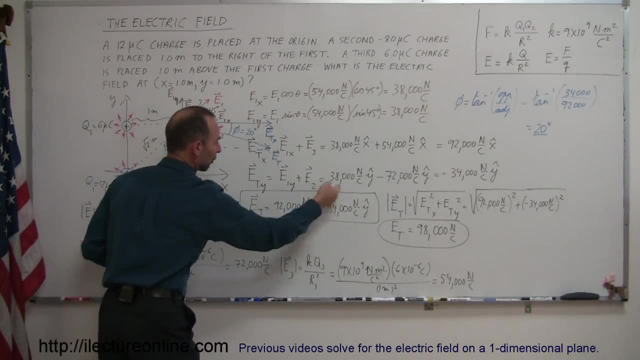 E total in the y is the y components of all the vectors that have y components. You get the magnitudes of the x and the y direction for the total vector, The total electric field, and you can write it here as a vector quantity or you can find: 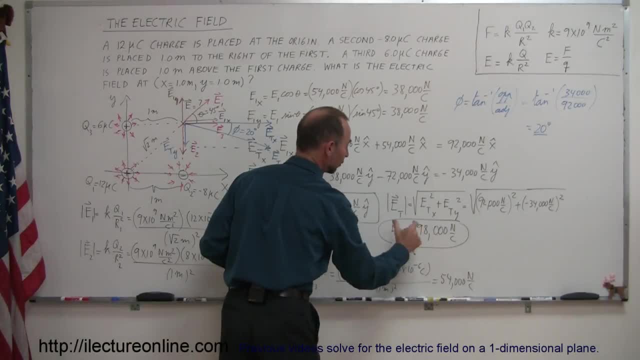 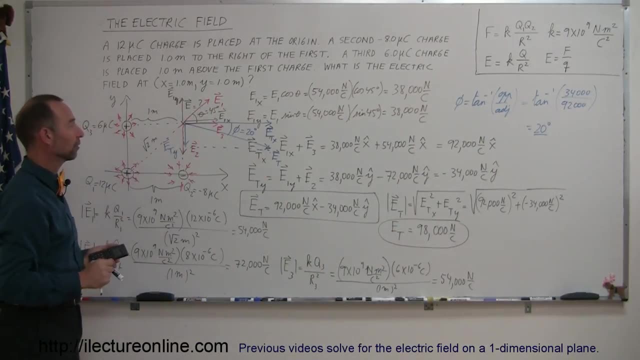 the magnitude of that using Pythagorean theorem right there to find the magnitude of the total vector and then find the angle relative to one of the axes. In this case, we found the angle relative to the positive x axis, And there's a little summary of how to do a problem like that. 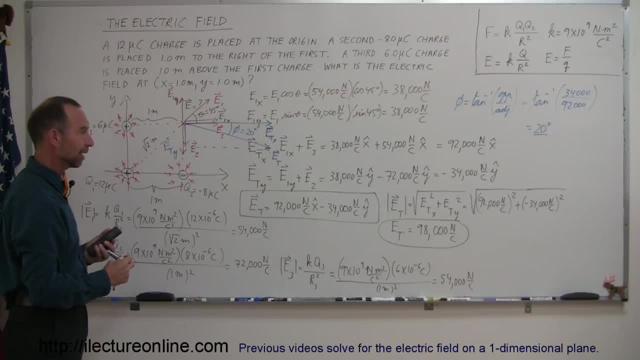 Go ahead and give that a try, See if you can duplicate this And don't get frustrated. Take your time. This can get quite complicated. All right, Good luck. 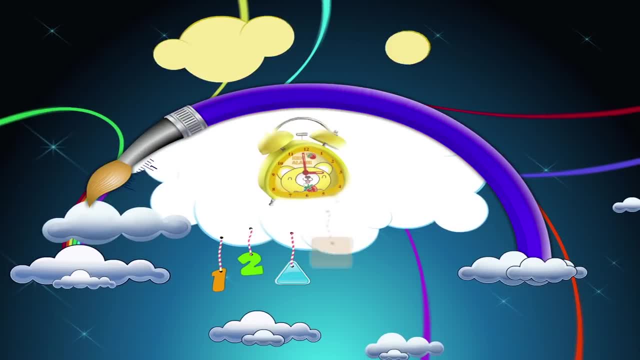 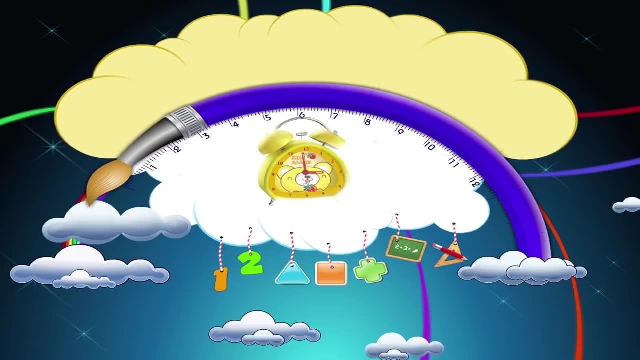 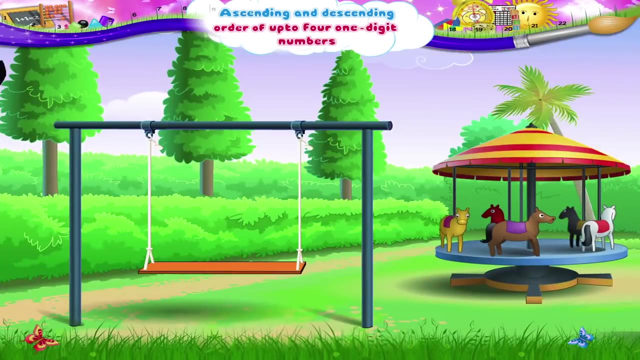 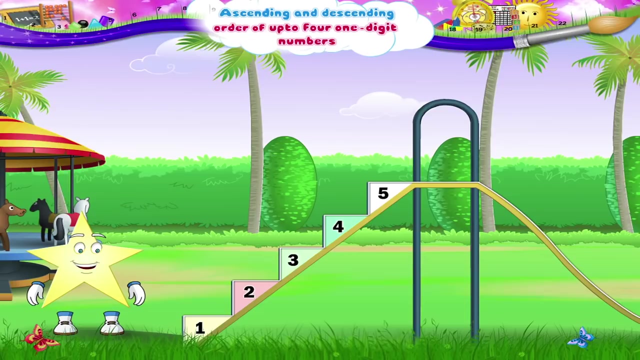 Ascending and descending. order of up to four one-digit numbers. Starry, here we are at the park. So many things to play on: Swings, merry-go-rounds. Oh, I'm sure you like this slide the best. It has colourful steps with numbers on it.